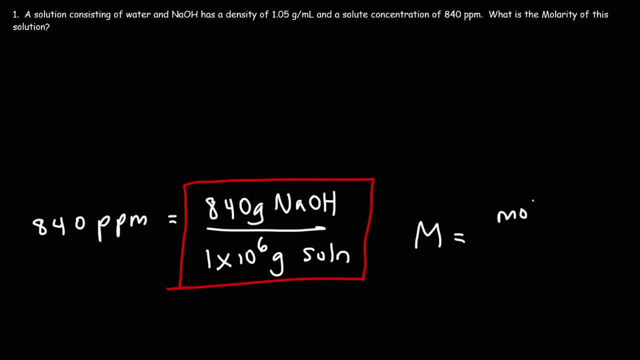 Now keep in mind: molarity is equal to the moles of solute divided by the liters of solution. So in order to convert from ppm, we need to convert from grams of solute to moles of solute, And we need to use the molar mass of NaOH to do that. 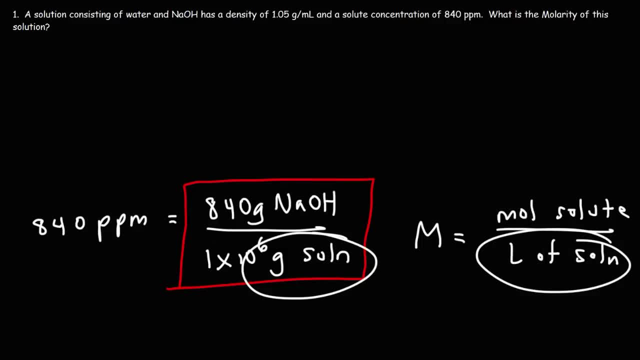 Now, to convert from grams of solution to liters of solution, we need the density of the solution. So that's how we're going to convert from grams of solution to liters of solution. So let's begin, Let's start, with this information: Our solution concentration. 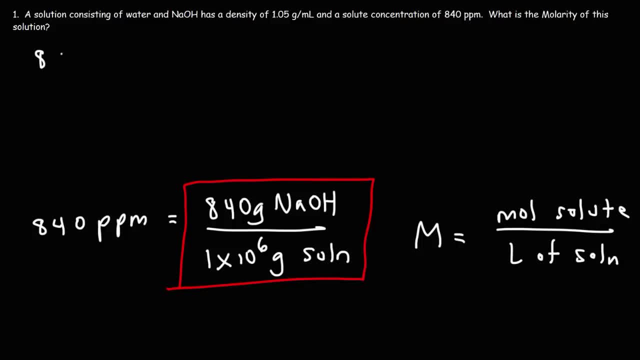 So instead of writing 840 parts per million, we're going to write 840 grams of sodium hydroxide per 1 million grams of solution. Okay, Now let's convert from g to b, Let's convert from grams to moles, So we need the molar mass of sodium hydroxide. Thus we need to add the atomic. 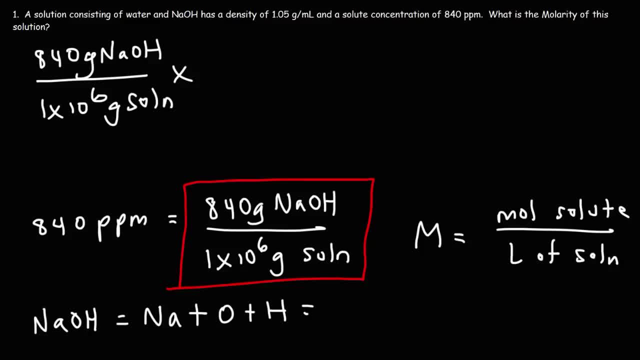 weights of each of the three elements using the periodic table. So according to the periodic table, the atomic weight of sodium is 22.99.. The atomic weight of oxygen is 16 and for hydrogen it's 1.008.. So 22.99 plus 16 plus 1.008, that's going to be 39.998.. But since 840 is such a 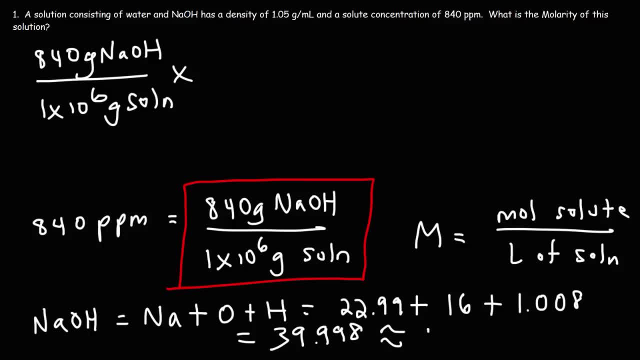 a nice round number. let's round the molar mass to 40.. So it's 40 grams per mole. So what this means is that one mole of sodium hydroxide has a mass of 1.008.. So that's going to be 1.008.. So let's round the molar mass to 40. So it's 40 grams per. 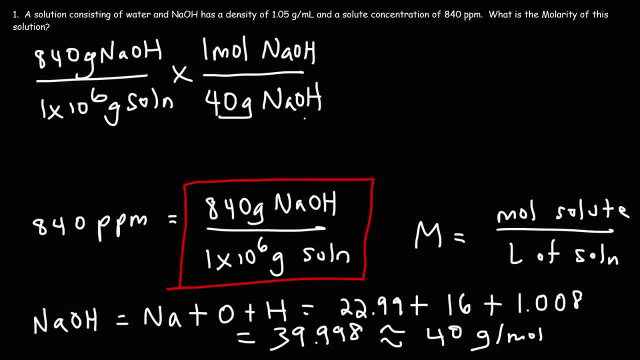 mole. So now we can cancel the unit grams of NaOH. So we have the first part. We now have the moles of solute. Now we need to use the density of the solution to convert from grams of solution to some unit of volume. The density is 1.05 grams per milliliter, So this means that 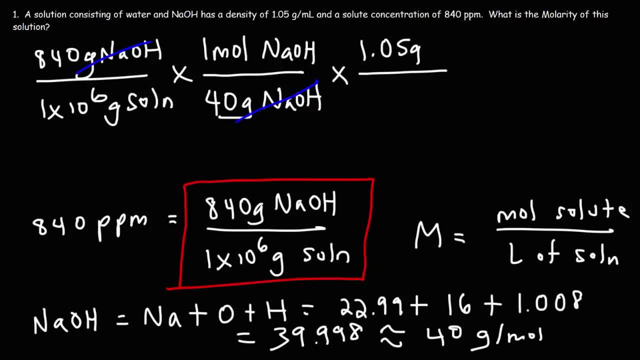 1.05 grams of solution is equal to or equates to a volume of one milliliters of solution. So now we can cross out grams of solution. Now what we need to do is we need to get liters of solution, So we need to convert from milliliters to liters. One liter is equal to one. 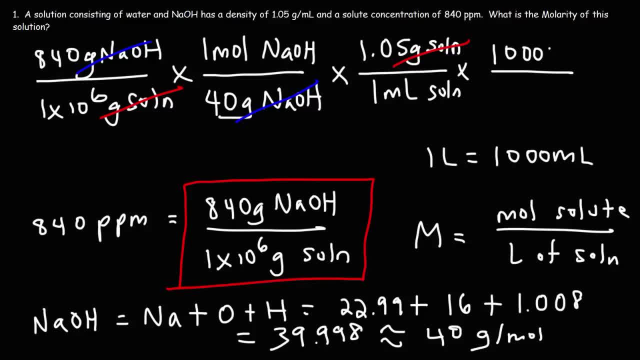 thousand milliliters. So we can put a thousand milliliters on top and one liter of solution on the bottom. So now we can cross out milliliters. So this is going to give us our answer, because we now have the moles of solute divided by the liters of solution. So let's do the math. So it's going. 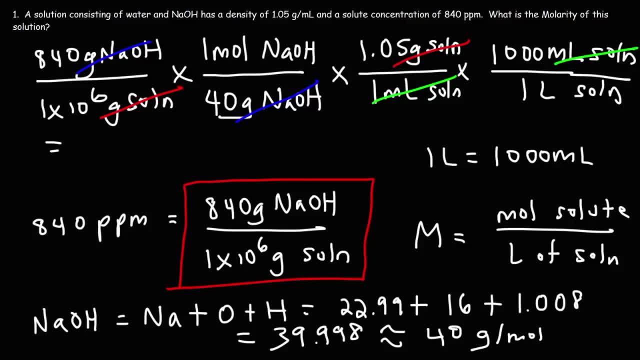 to be 840 divided by 1 times 10 to the sixth, And then take that divided by the liters of solution, Divide it by 40. And then multiply that by 1.05 times a thousand. So basically you need to. 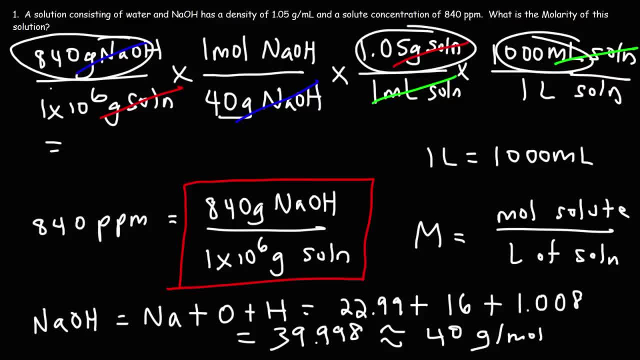 multiply by all of the numbers on top and divide by the numbers on the bottom. So the answer that I got is 0.022 m or 0.022 moles of solute per liters of solution. So that's how you can go. 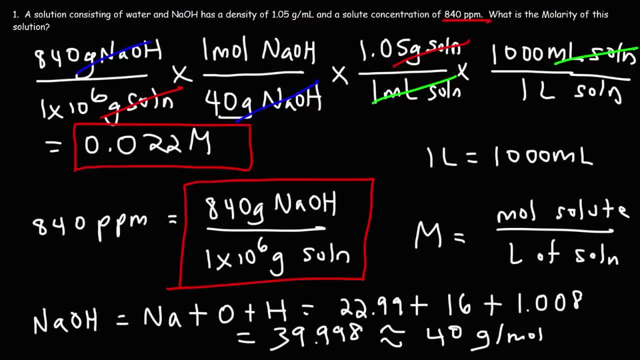 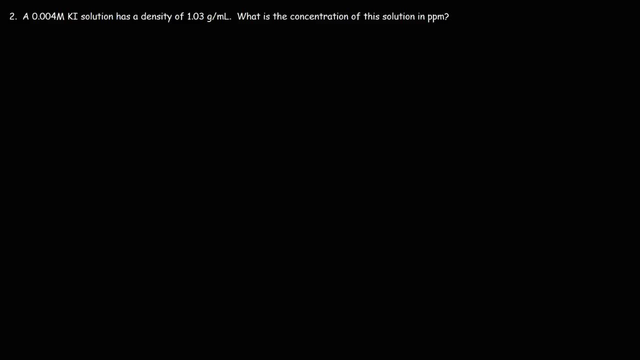 from parts per million to molarity. Now, what about working backwards? Well, let's try an example problem of how we can go back from molarity to parts per million. Number two: a 0.004 molar potassium iodide solution has a density of 1.03 grams per milliliter. What is the concentration of? 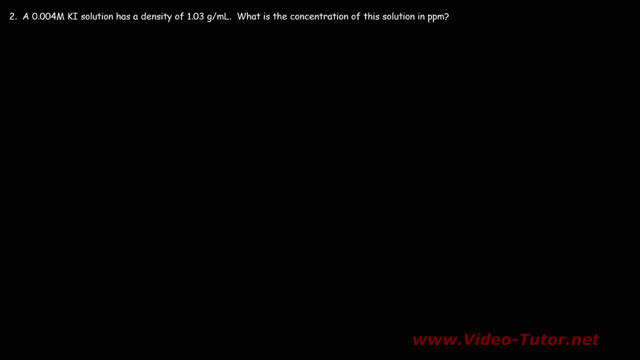 this solution in PPM. Now, if you want to pause the video and see if you can get the answer here, feel free to do so And then play the video when you're ready to see the solution. So go ahead, take a minute, grab a sheet. 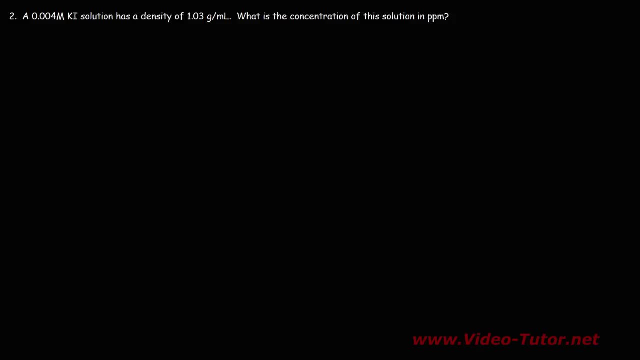 of paper and try this problem. So what we're going to do is we're going to start with the units of molarity, But we're not going to write it as 0.004 m, because molarity is moles of solute per liter. 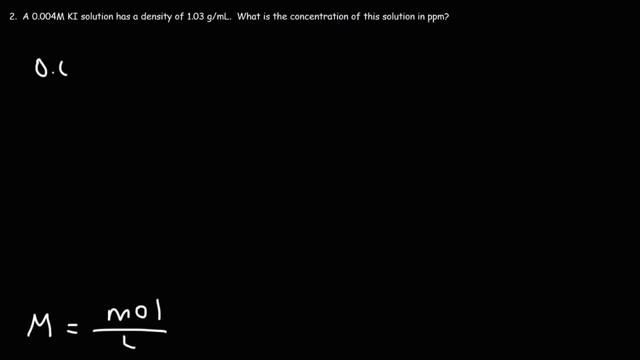 So we're going to write it as 0.004 moles of Ki per one liter of solution. In our next step, we're going to convert from moles of Ki to grams of Ki, And in order for us to do that, we need the molar. 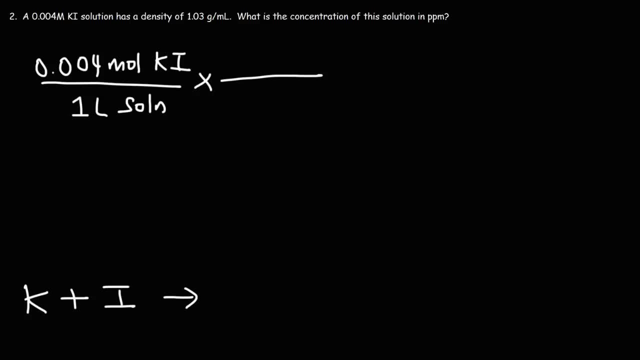 mass of Ki. According to the periodic table, potassium has an atomic mass of 39.1.. Iodine has an atomic mass of 126.9.. Adding these two numbers together, we get a molar mass of 166 grams per mole. So one mole of Ki has a mass of 166 grams. So 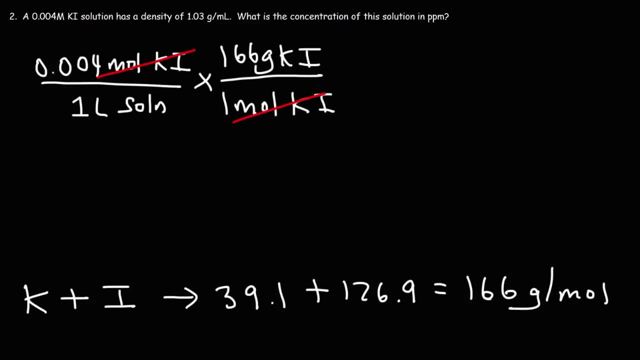 that's the first step, And then we're going to convert from moles of solute to grams of solute. Now remember the parts per million formula is grams of solute divided by grams of solution, times 10 to the sixth, So in: 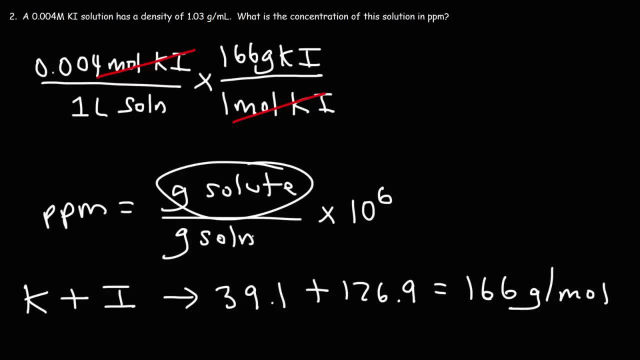 this conversion process. we need to get these two things. We already have grams of solute on top, as we could see here, So the first part is complete. The next thing we need to do is get the moles of solute on top of theumbs, or at least- 뭣o, I'm truthfully saying- the moles. 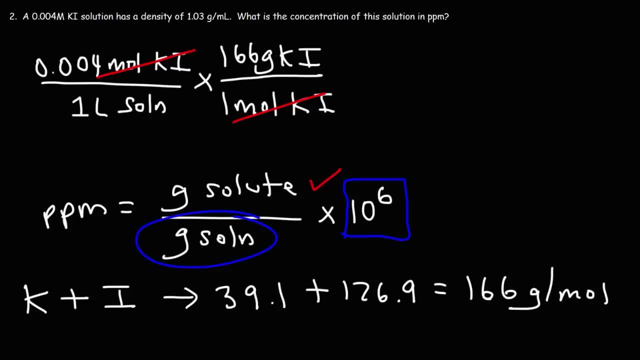 of solution on the bottom. Once we have that, we're just going to multiply whatever we have at that point by 10 to the sixth. So I'm just going to keep that there for now. So what we need to do is convert leaders of solution to grams of solution. That's what we need to focus on And we can use it density to do that. But we got to convert leaders of solution having as many resource too. The dessine. 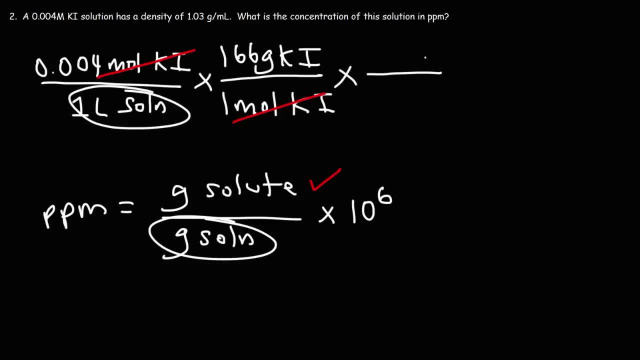 milliliters, and we know that one liter is equal to a thousand milliliters. so now this disappears. now that we have the volume in milliliters, we can now use the density of the solution. so one milliliter of the solution has a mass of 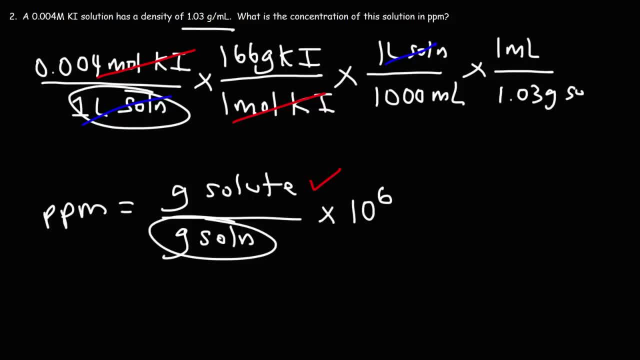 one point zero three grams of solution. now we have the grams of solute, which is good, but we also have the grams of solution on the bottom. so now that we have grams of solute over grams of solution, all we need to do is multiply the that result by 10 to the 6. so we're going to add 10 to the 6 at the end. so 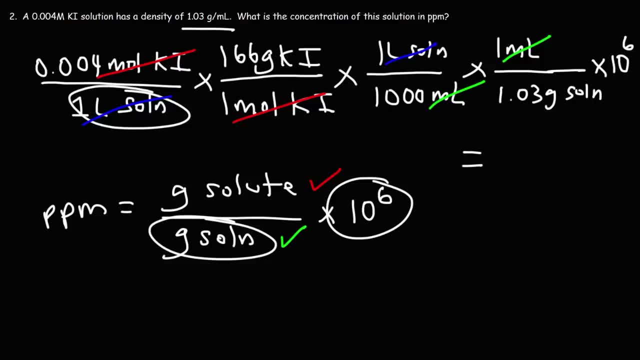 now let's do the math. don't forget we need to multiply by the numbers on top and divide by the numbers on the bottom. so it's going to be 0.004 times 166, and then divide that by a thousand, and then divide that result by 1.03 and then 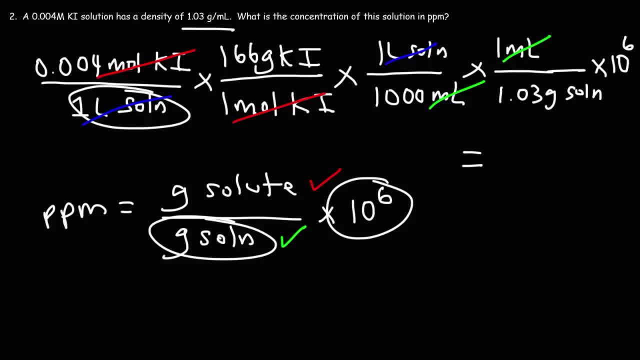 multiply it by 1 times 10 to the 6.. so you should get this answer. I'm going to write it over here: 644.7 parts per million. so this is the concentration of the Ki solution in ppm. so now you know how to convert from molarity to ppm. now let's say, if you want to convert from. 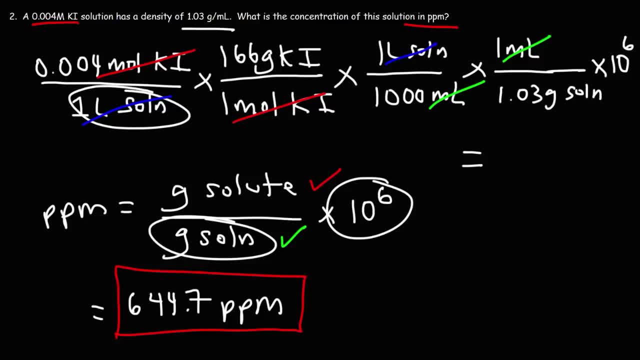 molarity to ppb. what would you do? it's important to understand that when you're doing the ppm test, you're going to have a solution concentration that is equal to one ppm is equal to a thousand parts per billion, so all you need to do is take. 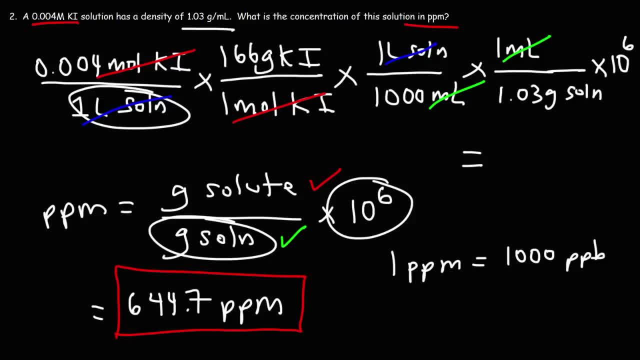 this answer and multiply it by a thousand and you can get the solution concentration in ppb. or, instead of using 10 to six, you could use tenth to nine and get the concentration in ppb, because the formula for ppb is: it's equal to the grams of solute divided by the mass of the solution in grams and the